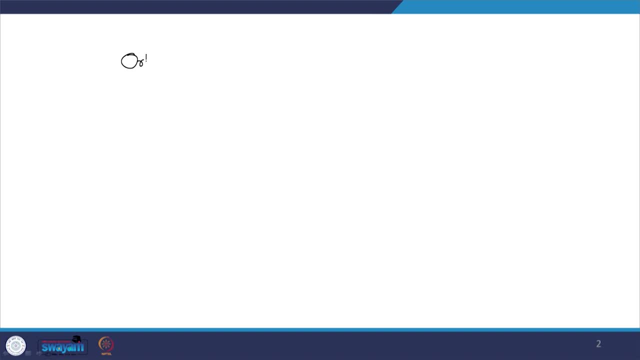 So what is orthogonal complement? Let V be an inner product space, let W be a subspace subspace, w be a subspace of B. The orthogonal complement of W is a set, is a subset, W complement of B, such that the 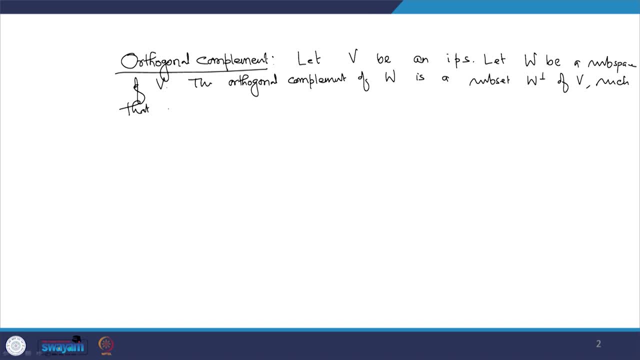 set. each element of W complement is orthogonal to every element of W. So this implies your W bar. I can say that this W bar, which is subset of B and W complement, is also a subspace of W, So W complement is a subspace of V. this has to be also prove it. 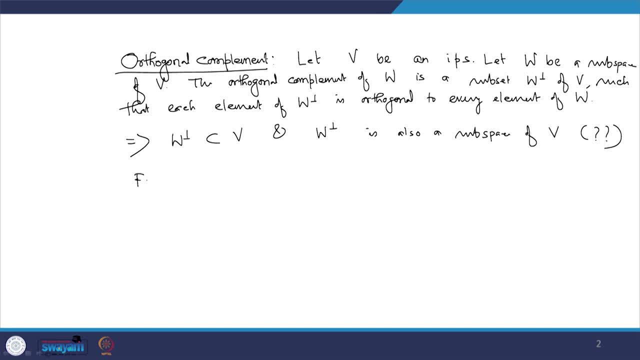 So for any alpha beta belongs to W bar W complement and C belongs to the field over which the vector space V is defined. Ok, Then claim C alpha plus beta also belongs to W complement. So this will be in W complement, provided C alpha plus beta is orthogonal to each element. 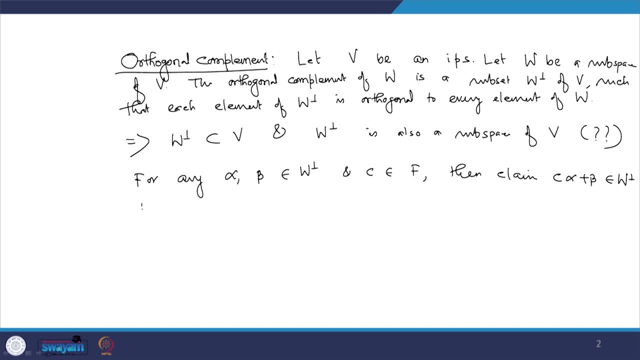 of W We have For, For any gamma belongs to W inner product of C, alpha plus beta and gamma is equal to C inner product of alpha gamma plus inner product of beta gamma. So since alpha belongs to W, complement and orthogonal complement. 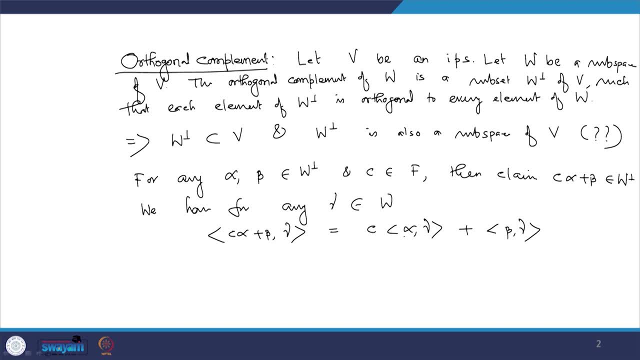 Ok, Ok, So then gamma belongs to W and alpha Rah shall be orthogonal to W. Yes, So then we are leaving it. Well, this is nothing but the diagonal Lindsay's revolutionary curve of 추 vest… Yes … So thisₚ is בח subscribedₛis equal to Q bumped integral eins and λ questo. 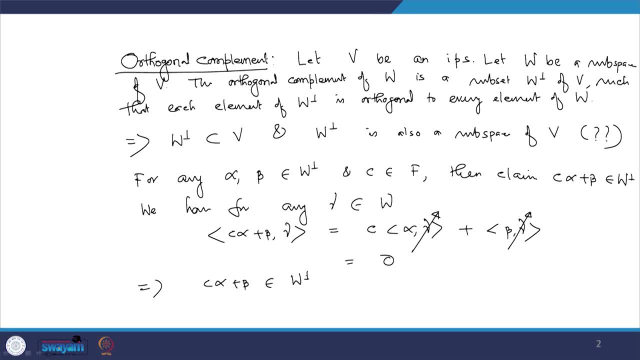 significa that this is equal to 0. this is also equal to 0. So staple. So this means that this is equal to 0, So this implies C. alpha plus beta also belongs here. the orthogonal complement of the subspace W is also a subspace of the vector space V. 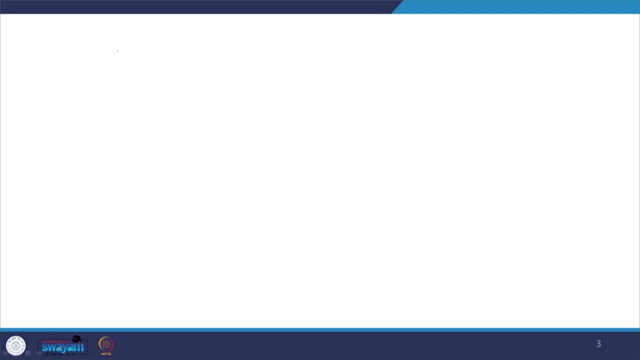 Let me introduce one more terminology. this is called orthogonal projection. So let V be an inner product space, inner product space, and W in this case is looking at the subspace. be a subspace of V. If for beta belongs to V, if the best approximation best approximation. 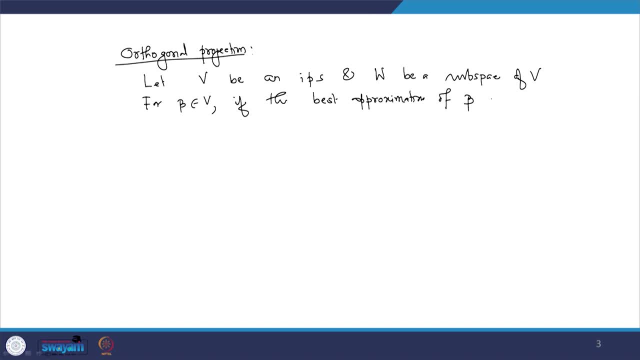 of beta on W exist. that is, if alpha belongs to W be the best approximation, then beta will be the best approximation. So if alpha belongs to W be the best approximation, then beta will be the best approximation. So alpha is called as orthogonal projection of beta. alpha is called as orthogonal projection. 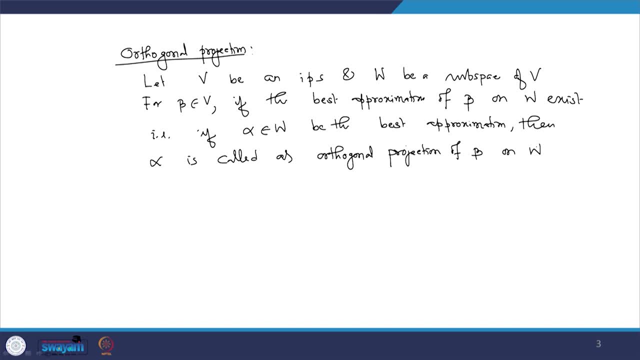 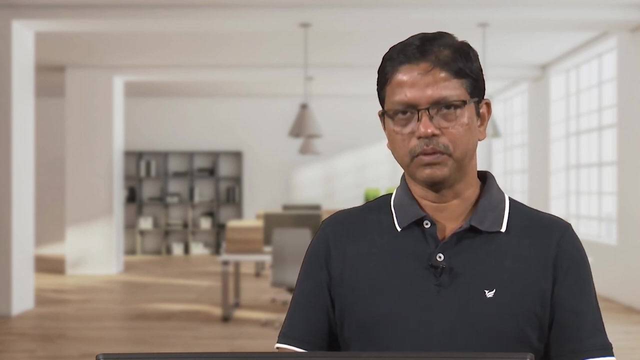 of beta on W, where we know that beta minus alpha is orthogonal to each element of W. See, in our last class we have seen: if W is finite dimensionals, then for each vector, beta in V, the best approximation of beta on W, exist and that is also unique, which is having 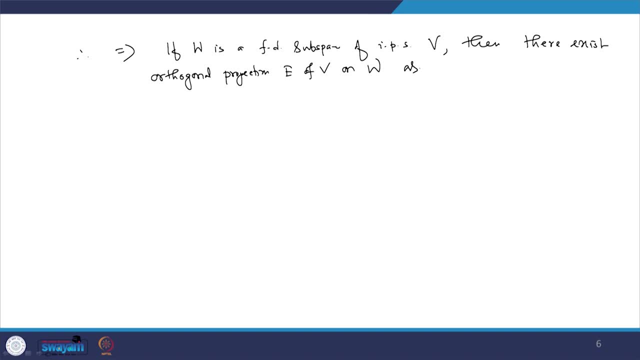 as as well as orthogonal projection of V on W complement, orthogonal complement, The way the orthogonal projection psi is defined. here the orthogonal projection psi is defined as theети python method And thisqf vector, that says the veil. 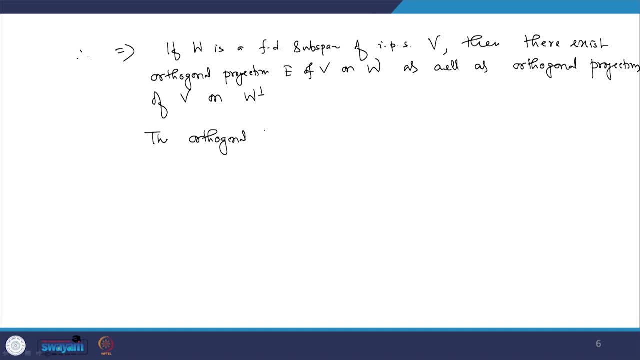 psi is basically, you know, i minus e, because psi of beta is equal to i minus e. operating on beta, that is equal to beta minus. So we have now seen that if V is an inner product space and W is a finite dimensional subspace of V, then there is a orthogonal position. 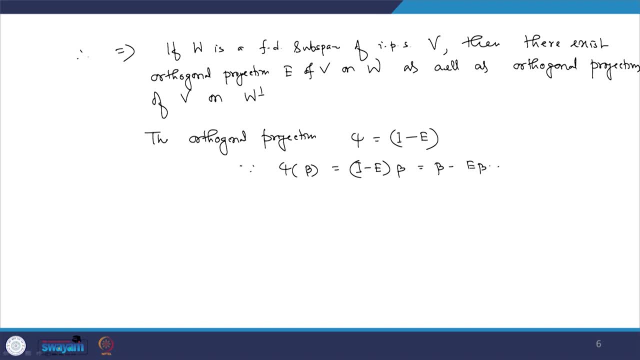 of V on W as well as on orthogonal complement of W. So this give a hints that is it possible to have a finite dimensional subspace of V? possible to write the space V as a direct sum of two subspaces which are independent to each other? So this questions can be answer by this theorems. 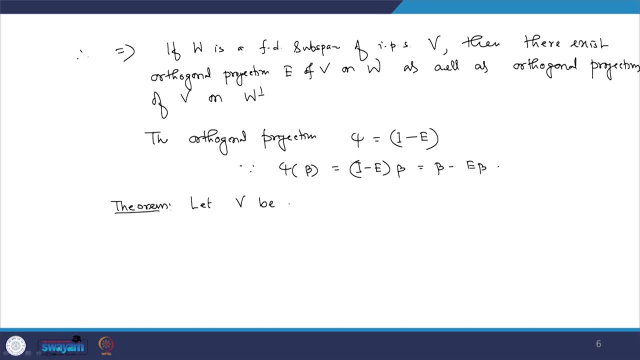 Let V be an inner product space. Let W be a finite dimensional subspace of V. Let E be the orthogonal projection of W. So this is the final answer. Let V be a finite dimensional subspace of V on W, Then E is an idempotent linear transformation. 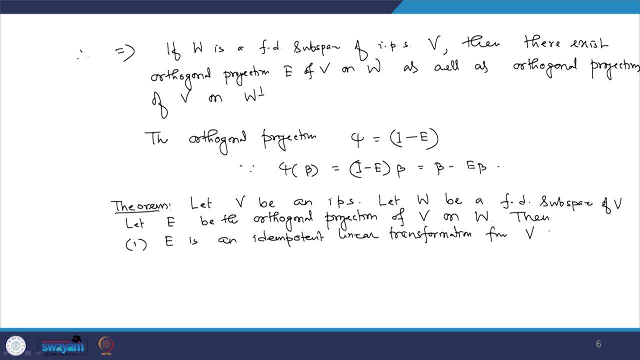 From V on to W, that is E square equal to E on W. Second, the null space of E is equal to W. So W is W complement, that is, orthogonal complement of W. Third, V is equal to direct sum of W and W complement. where W intersection, W complement equal to zero subspace. So let 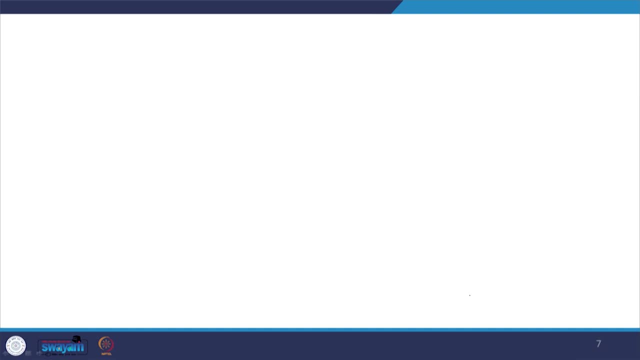 me prove one by one. this result is So. it is given. E is an orthogonal projection of V on W. So this implies E maps to any element. beta belongs to V to E beta, beta minus E beta is orthogonal to each element of W. Each element of this means E beta is the best. 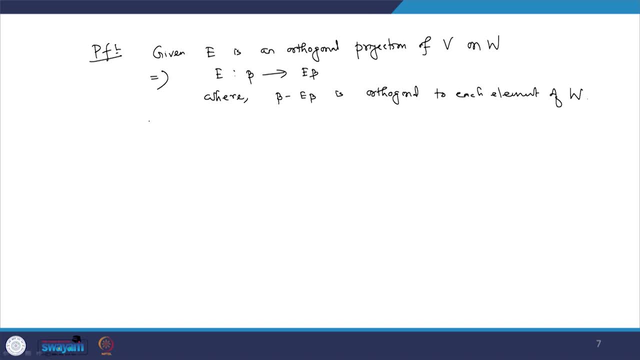 approximation of beta on W. So this implies if beta belongs to W, So certainly E beta will be equal to beta, So that the best approximation of beta on W will be itself. basically ok. So in this case, when you consider E operating on again, 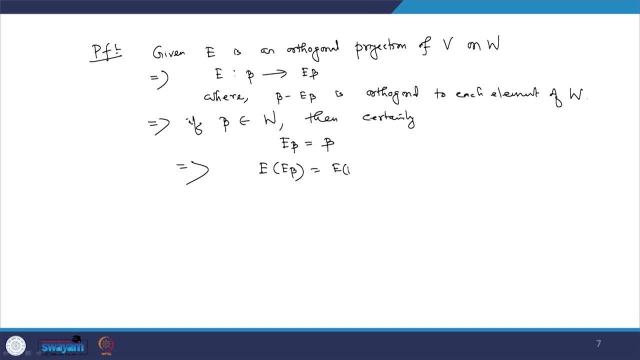 E beta. it is equal to E beta. So this implies that E square beta equal to E beta. this is true for all. beta belongs to W, So this implies E square equal to E. So this implies E is a important linear transformation from V onto W. So this is the first part of this results. 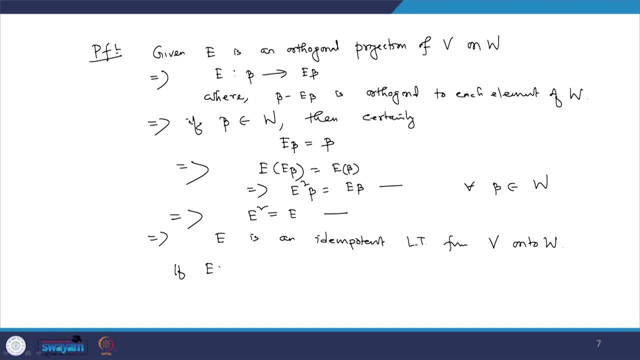 Second, if E of beta equal to 0, this implies that beta minus E of beta, which is equal to beta, is in W complement. So this implies that beta belongs to. So this implies E. beta equal to 0 implies beta belongs to the. I mean null space of beta. So this implies any element. 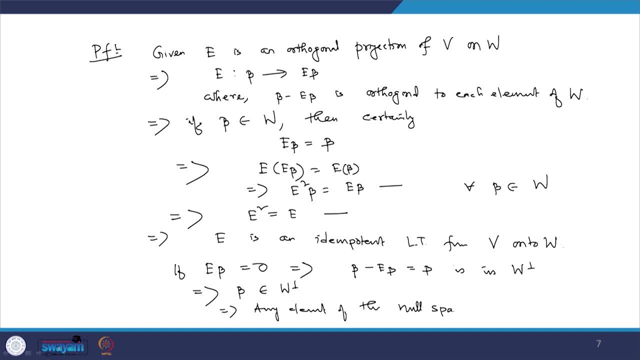 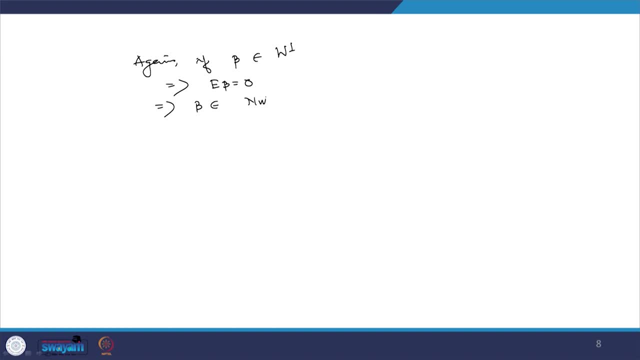 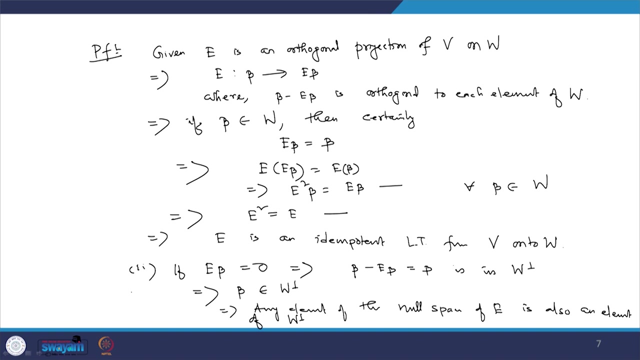 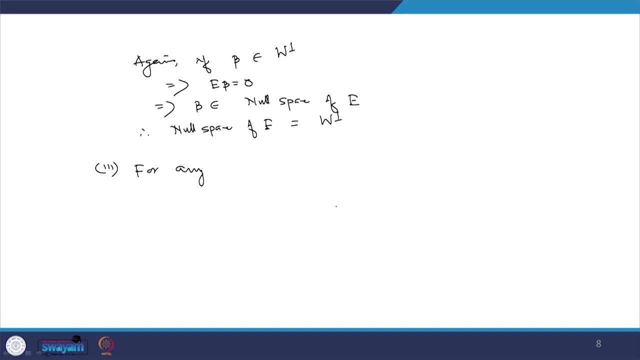 0. So this implies beta belongs to null space of E. So null space of E equal to W complement. Third, third one- this is my second and say first one. For third one that I have to show that V is the direct sum of W and W complement For this, for any beta belongs to V. we have 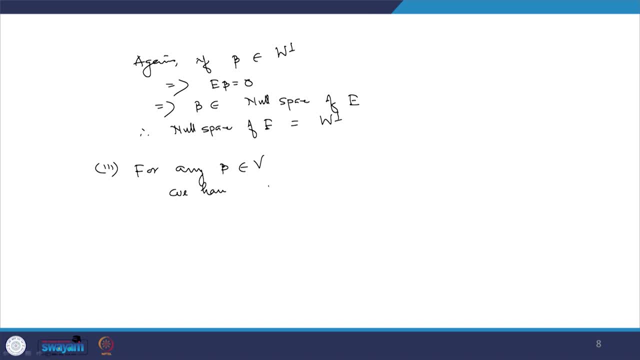 beta equal to E beta plus beta minus E beta. One can write down beta is equal to like this: So this implies E beta belongs to W and beta minus E beta belongs to W complement. So we see that beta can be written as the sum of element from the W and sum of as well. 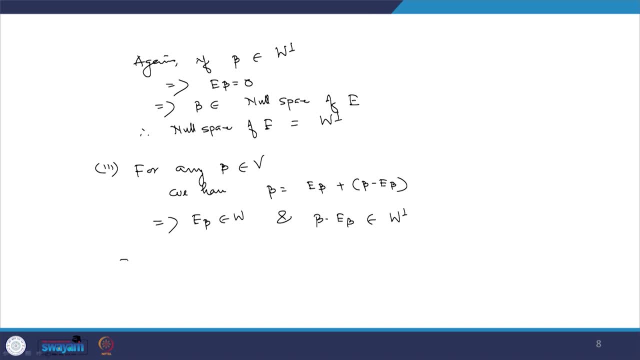 as element of the W complement place. So this implies beta can be written as as sum of element from W as well as E beta. So this implies element from your W complement. So it has two component: one component from W, another component from the W complement. It will be direct sum provided, if I can somehow. 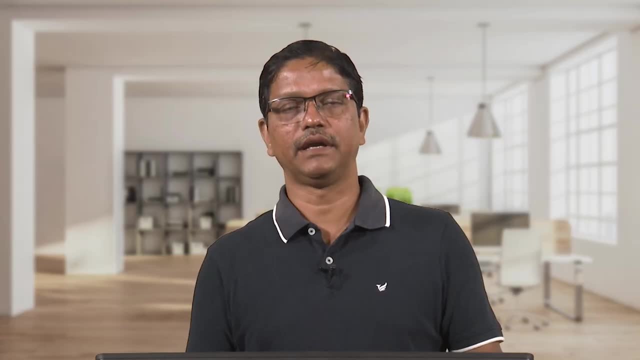 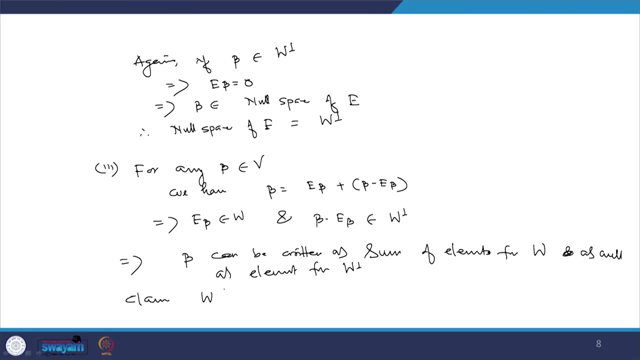 show that W and W complement. they are mutually disjoints. So now I want to show W intersection, W complement. equal to 0, subspace, Suppose, not if 0, not equal to alpha, belongs to W intersection, W complement. So this implies inner product. 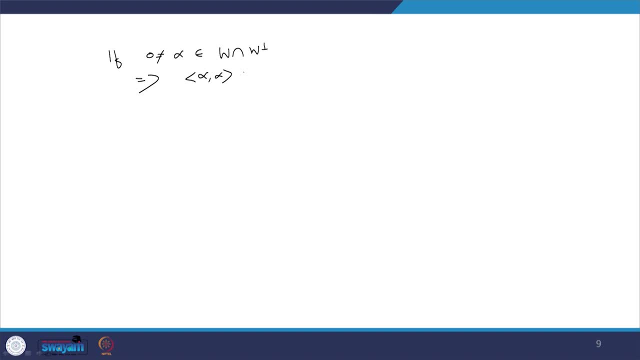 of alpha and alpha equal to 0.. Since alpha belongs to W, and so this implies alpha is orthogonal complement of itself, So this implies inner product of alpha and alpha equal to 0.. This is possible only when alpha equal to 0. 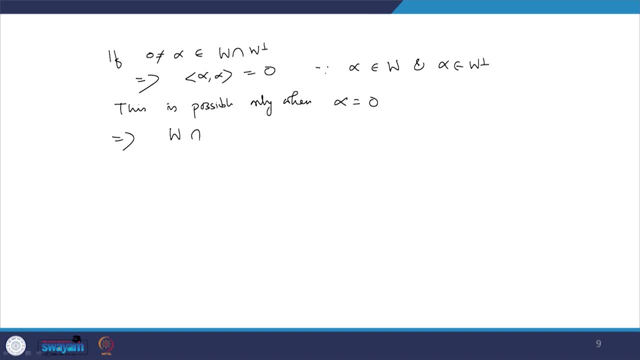 So this implies? So this implies that W intersection, W complement equal to 0 subspace. So now we have seen that if V is an inner product space and W is a finite dimensional subspace, then V can be written as direct sum of W and its corresponding orthogonal complement. So this given hints. 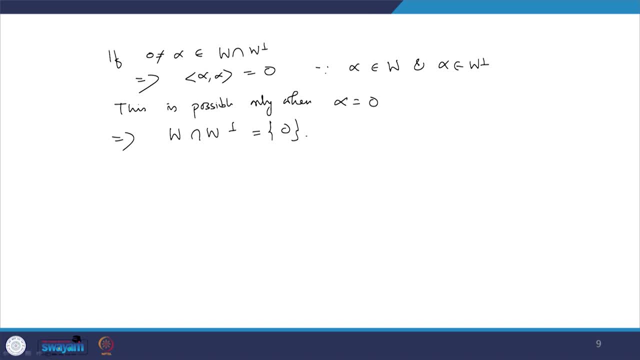 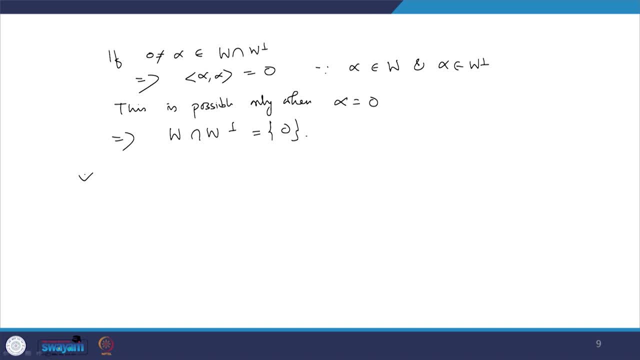 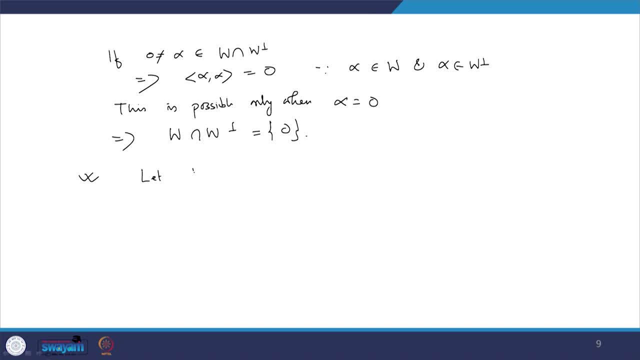 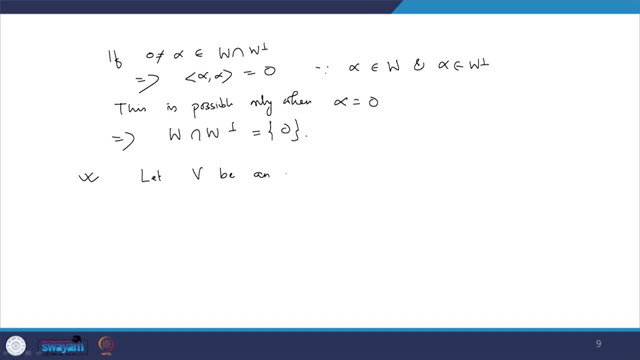 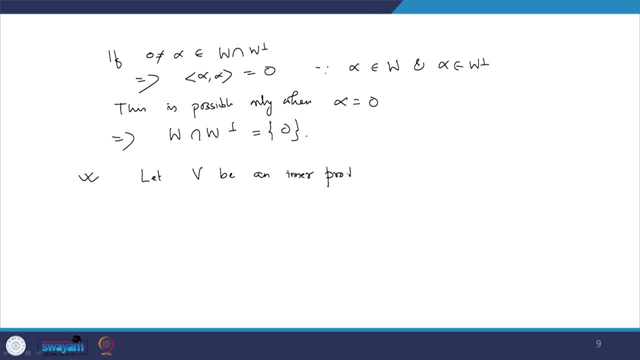 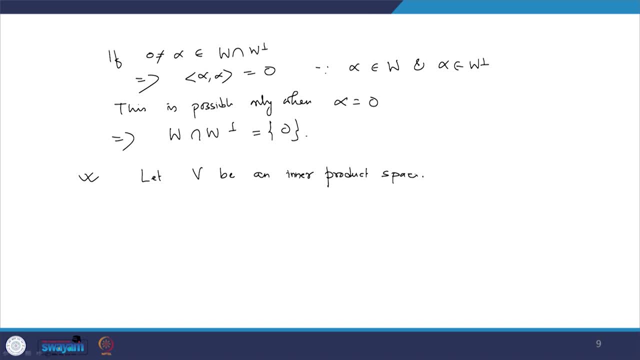 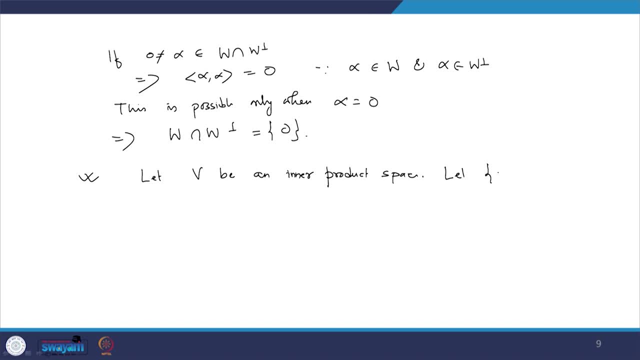 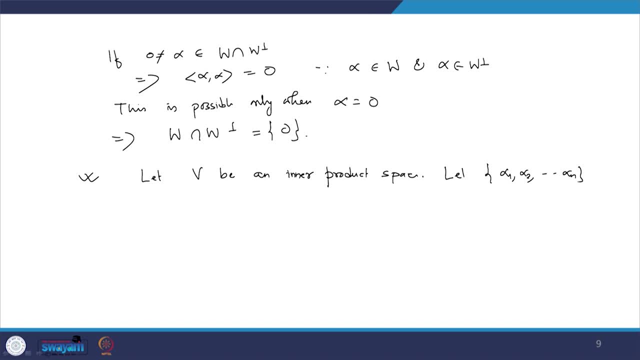 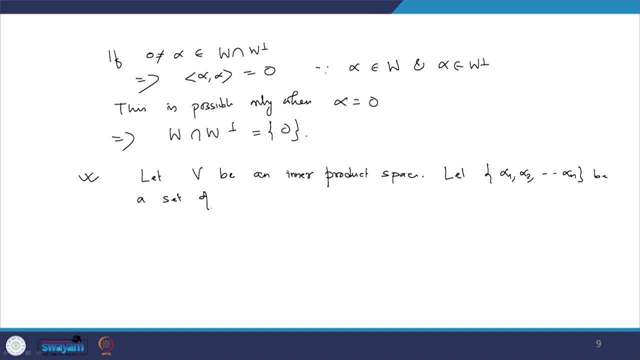 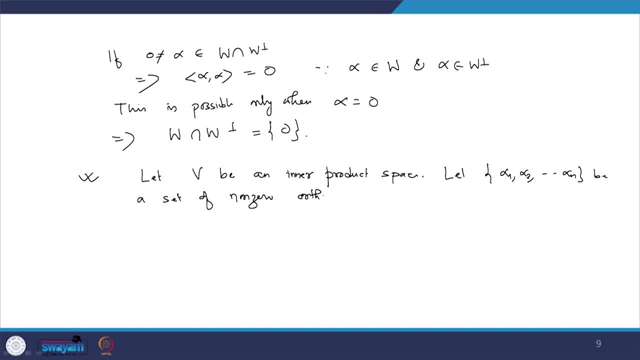 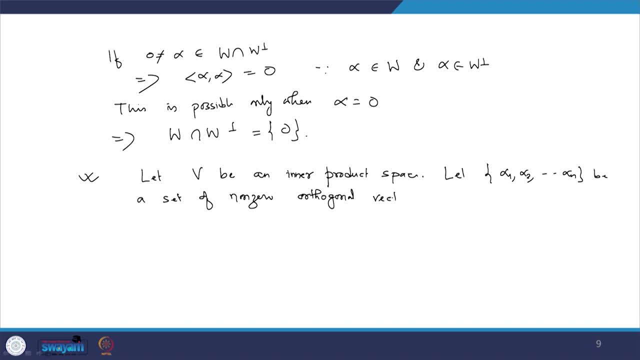 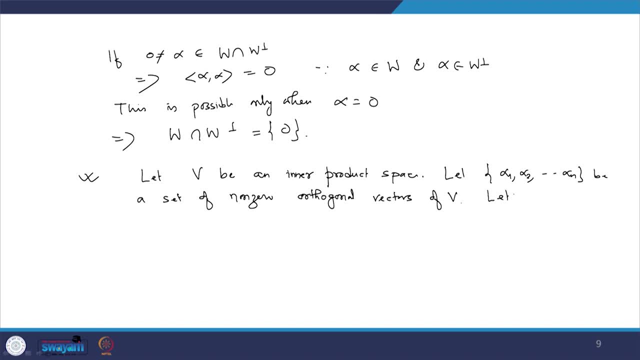 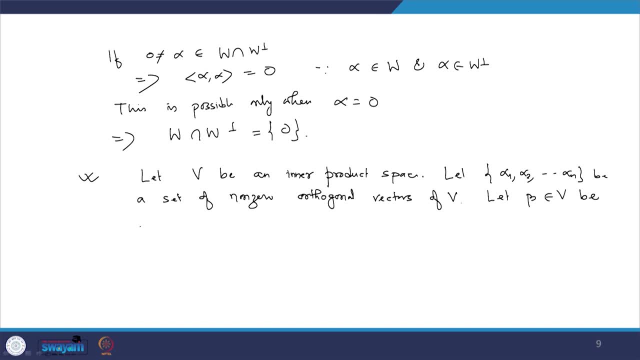 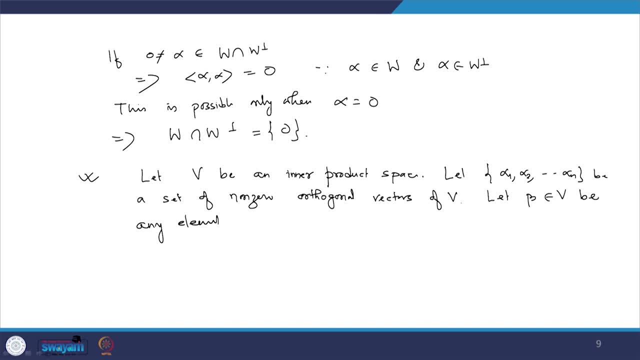 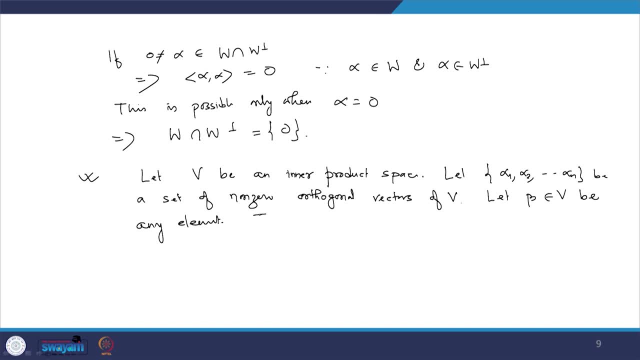 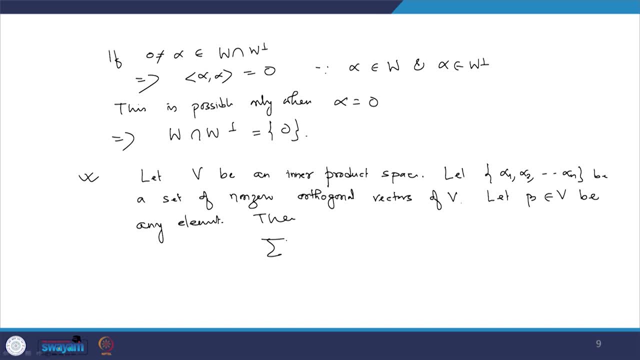 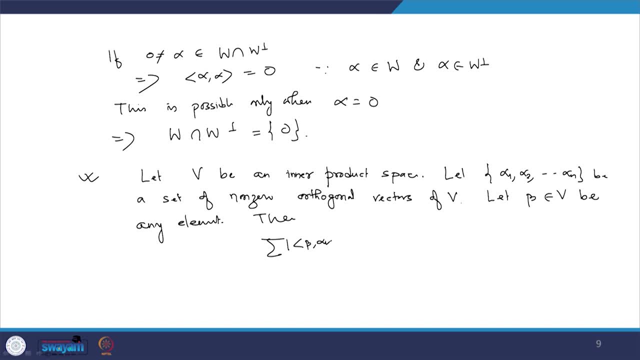 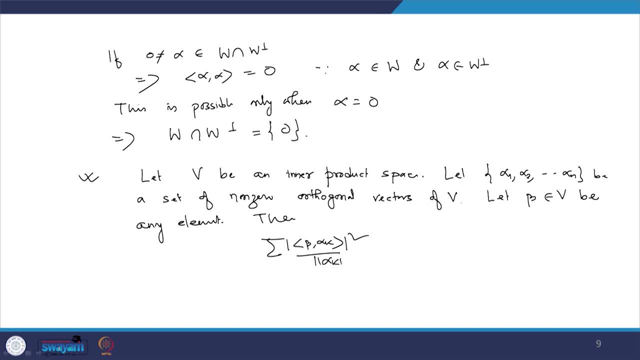 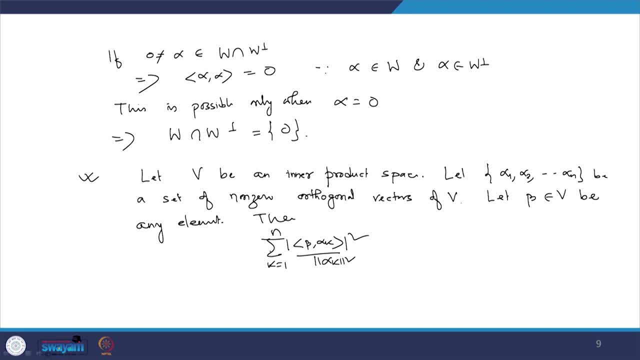 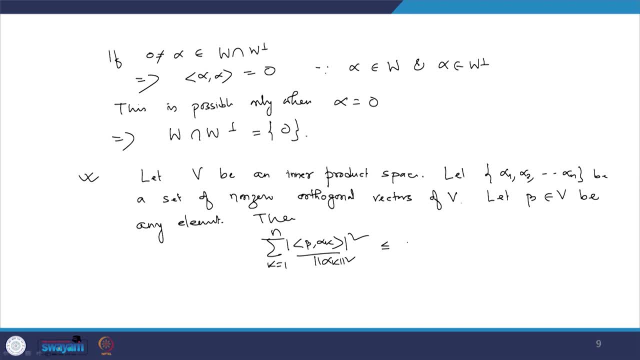 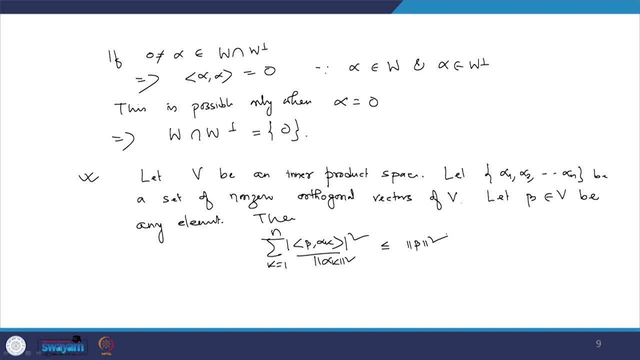 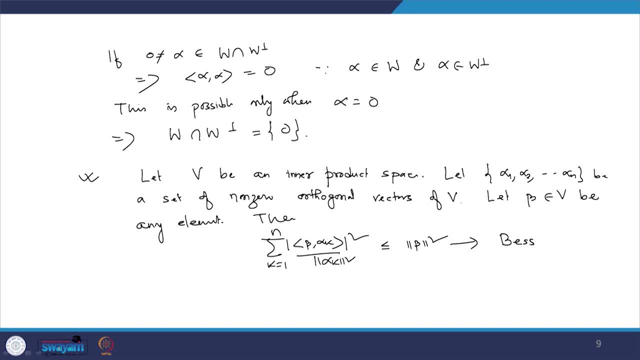 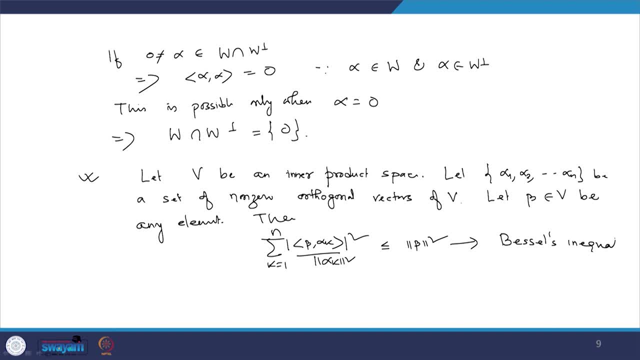 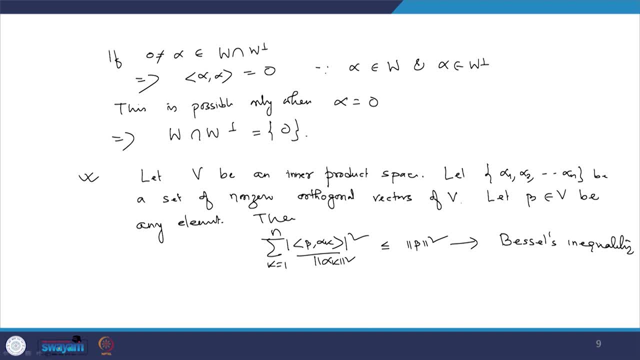 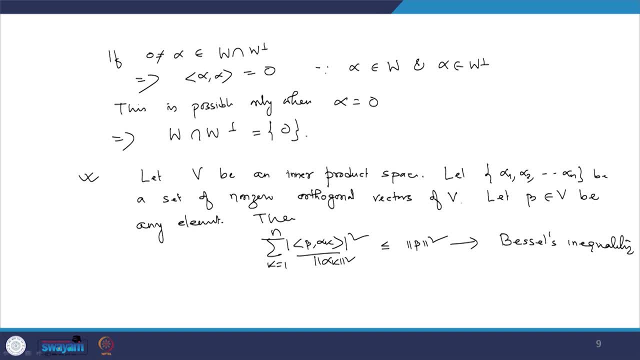 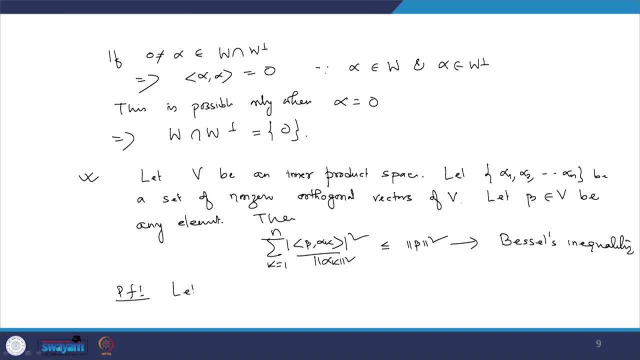 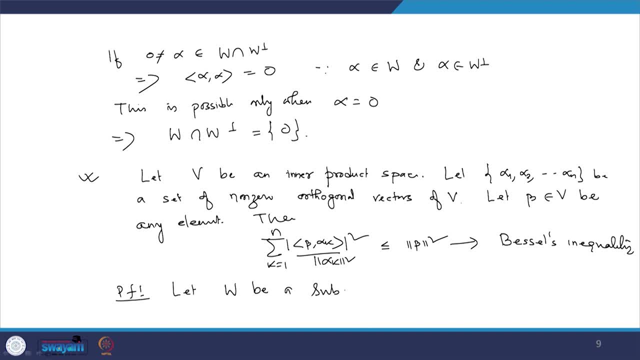 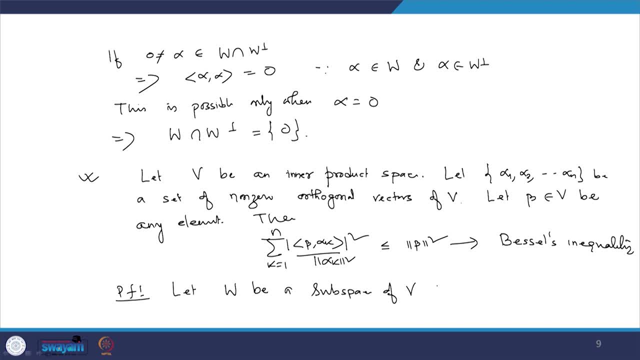 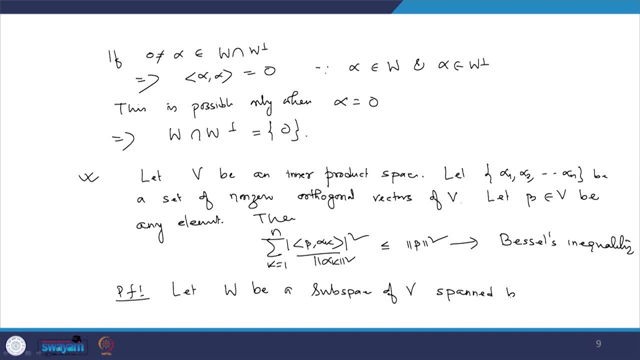 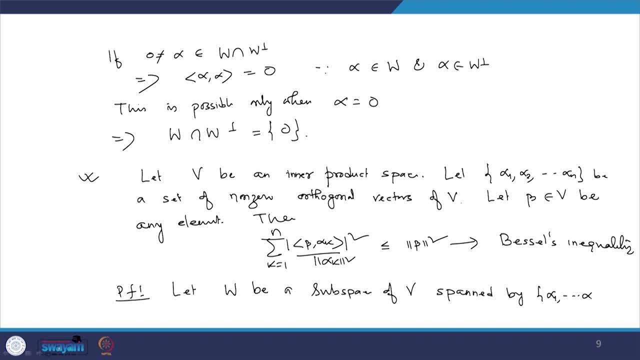 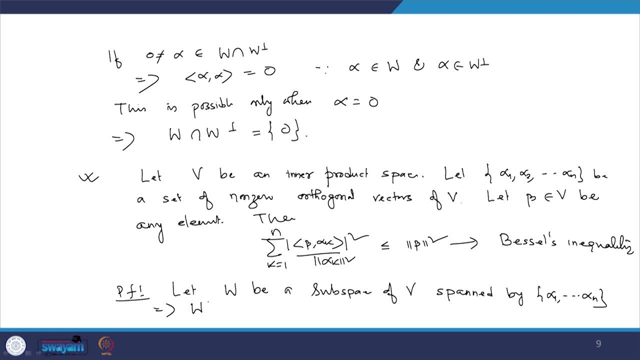 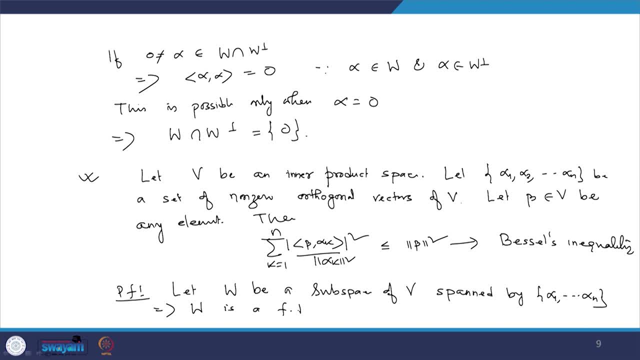 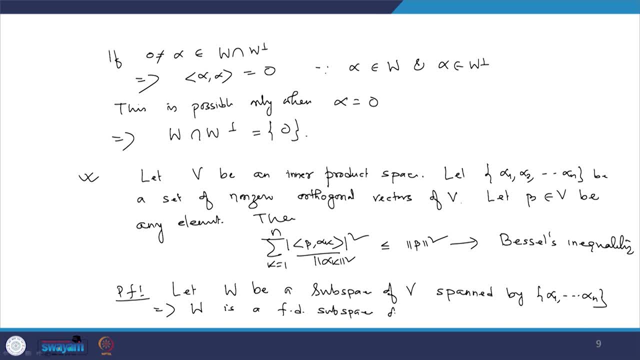 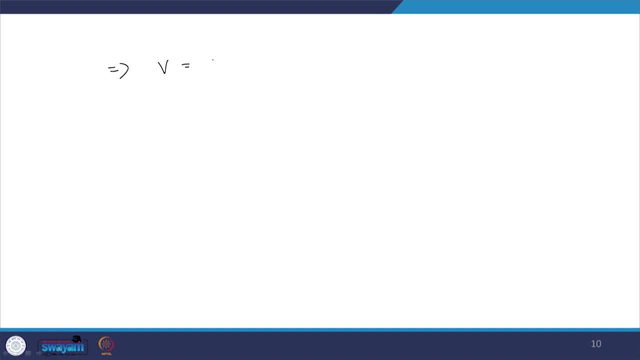 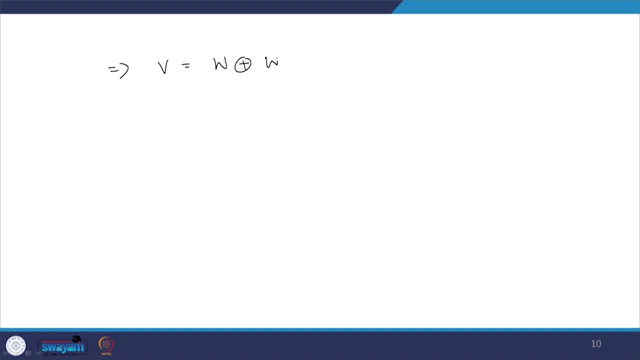 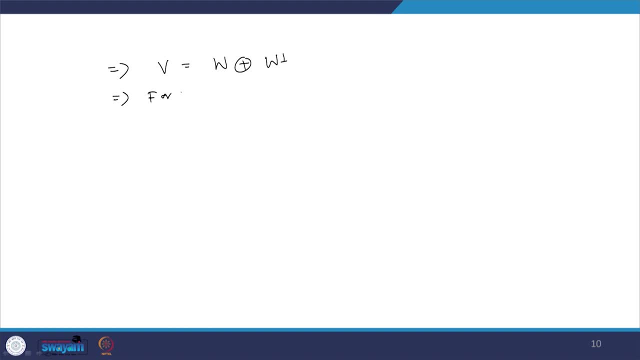 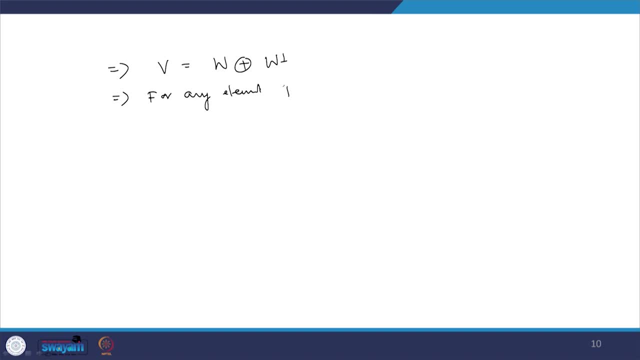 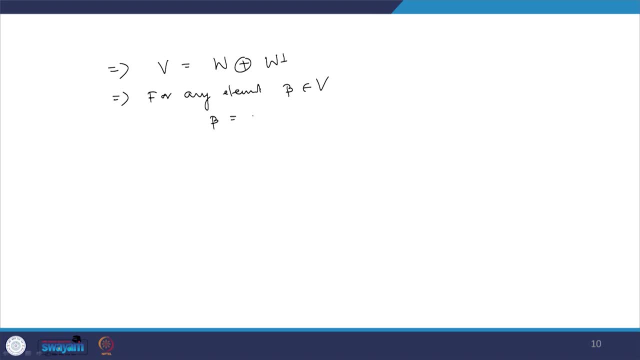 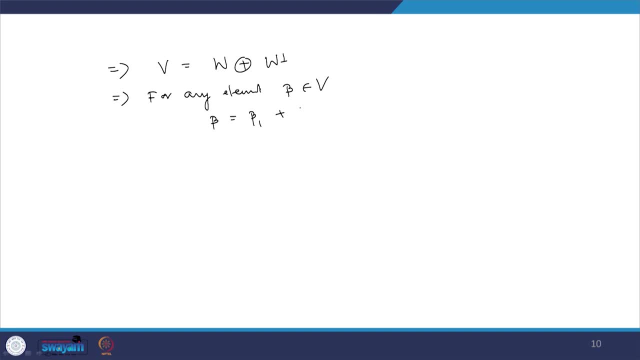 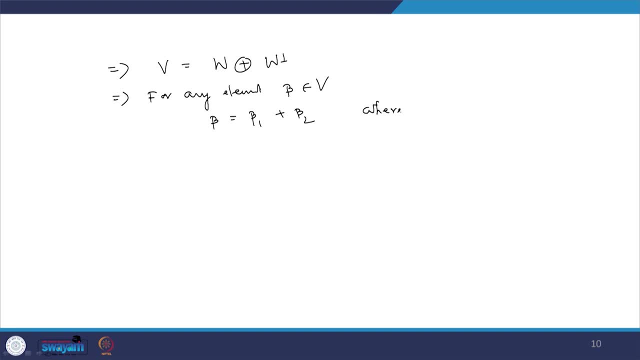 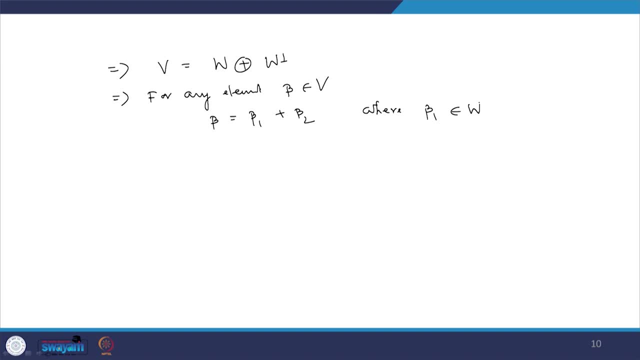 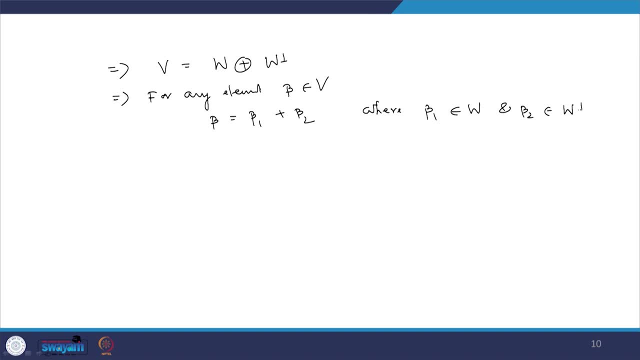 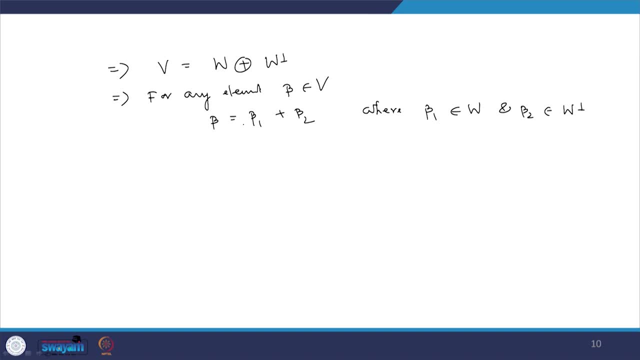 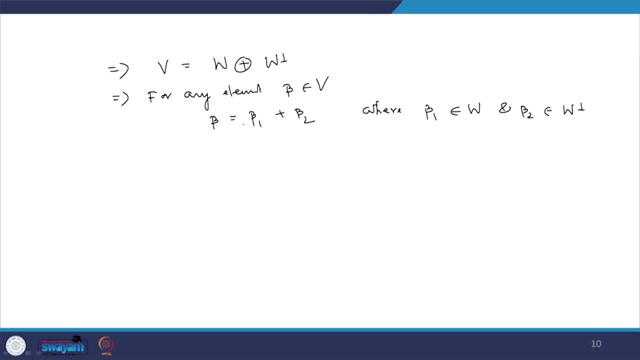 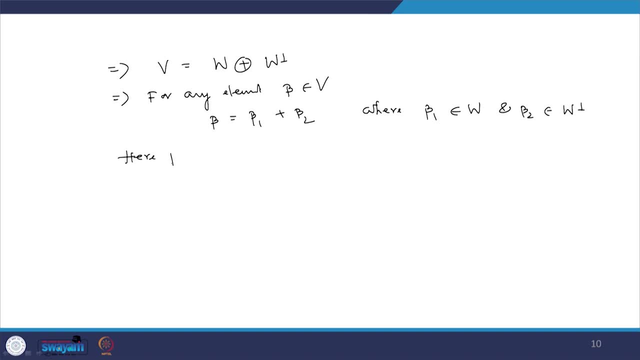 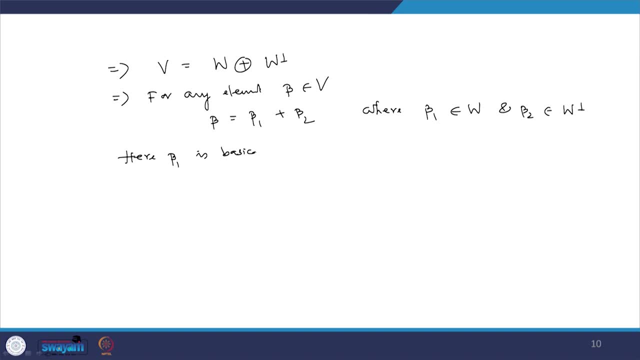 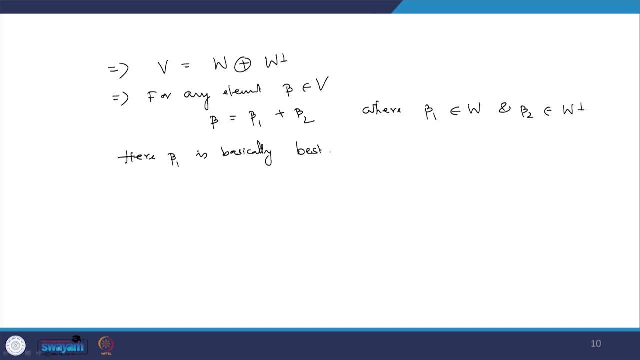 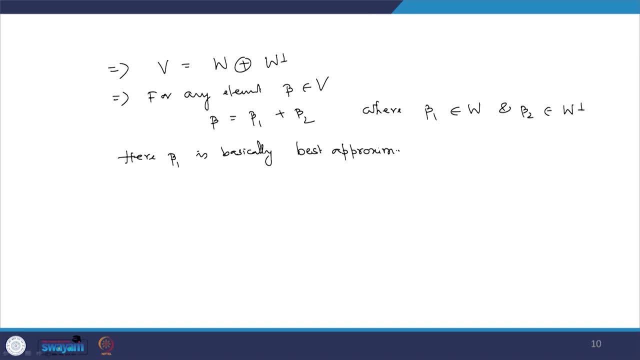 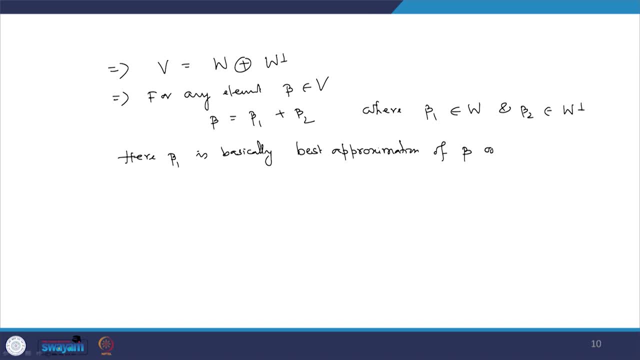 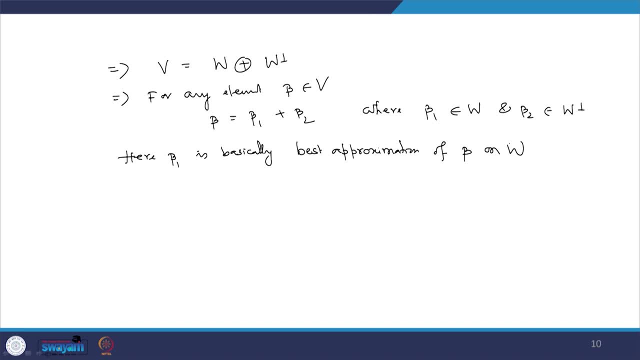 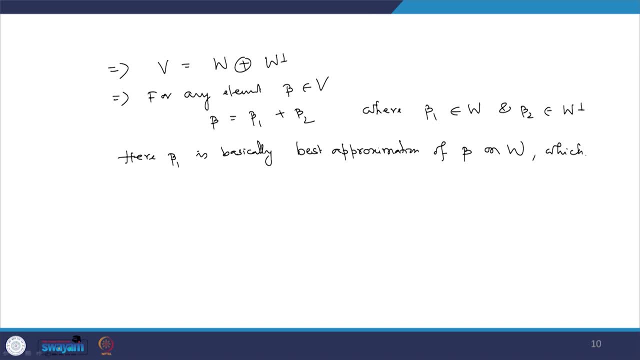 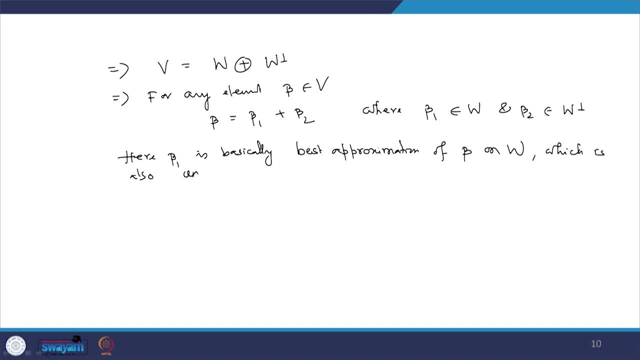 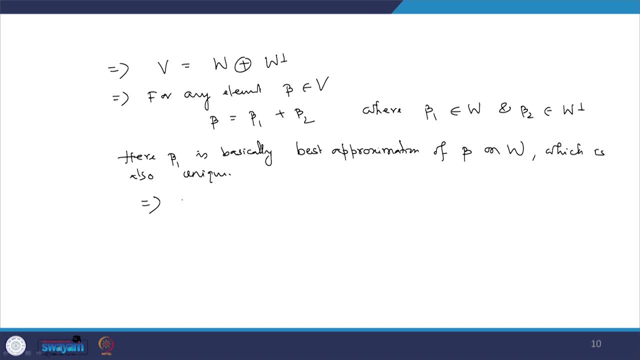 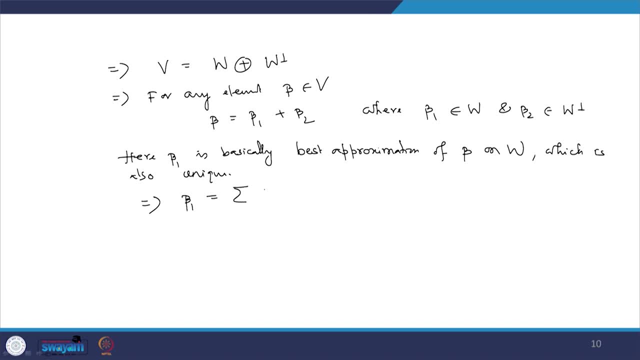 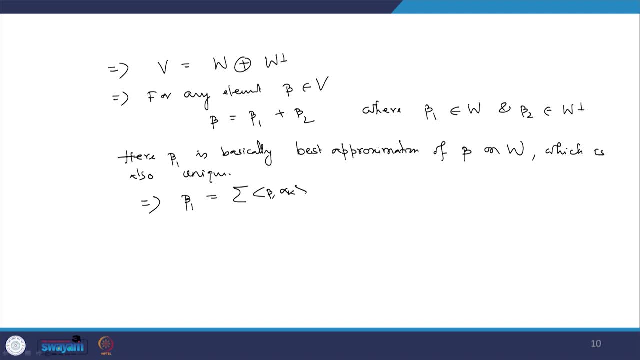 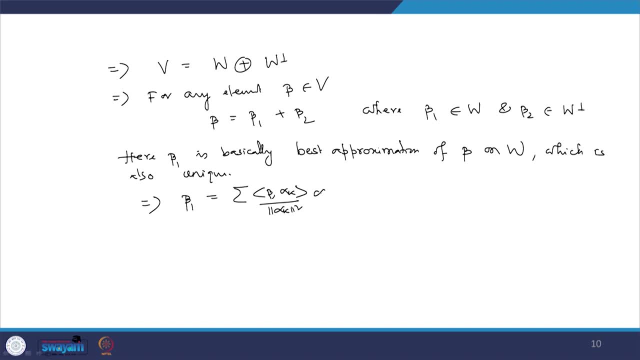 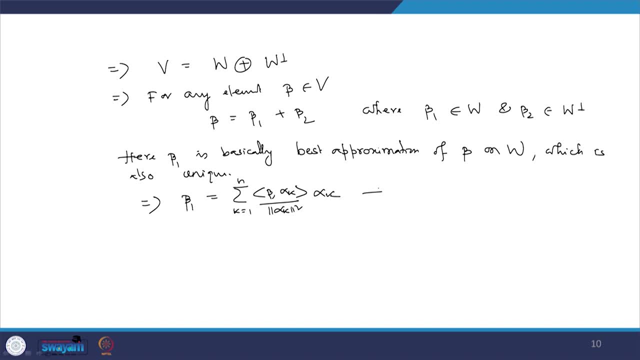 k, k equal to 1 to n, So I can have: beta 1 is like this thing: This is the best approximation of beta on W. So this implies that beta 1 is orthogonal to beta 2, also Now norm of. 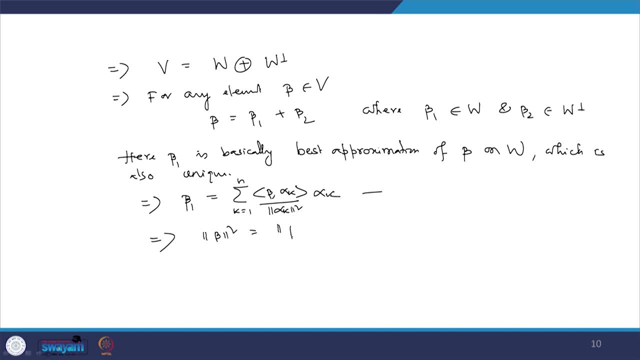 beta square is equal to norm of beta 1 plus beta 2 square. So this is equal to, basically, norm of beta 1 square plus norm of beta 2 square, since inner product of beta 1 and beta 2 equal to 0. So you have norm of beta square equal to. like this, Beta 1 square is: 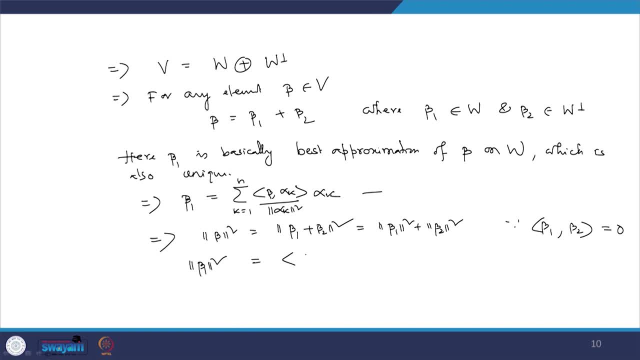 nothing inner product of sigma beta alpha k by beta 1 square By norm of alpha k square and alpha k and sigma beta alpha, j suppose, by norm of alpha j square and alpha j. For sake of simplicity only, I have changed the suffix so that it will. 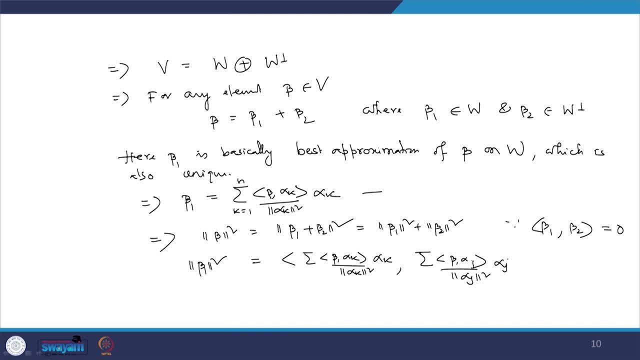 be it will not confuse us that why we have written same alpha j. So I can say j equal to 1 to n, k equal to 1 to n. So if I use the basic definition of inner product, then this is going to and use the orthogonality nature of alpha i. So this will give me basically: 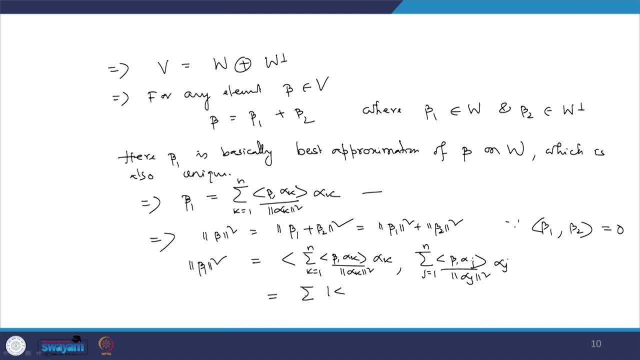 your sigma amount of beta and alpha k square by norm of alpha k square only k equal to 1 to n, So you can check as a homework that this is correct. This implies norm of beta square is equal to sigma inner product of beta and alpha k square by norm of alpha k square. 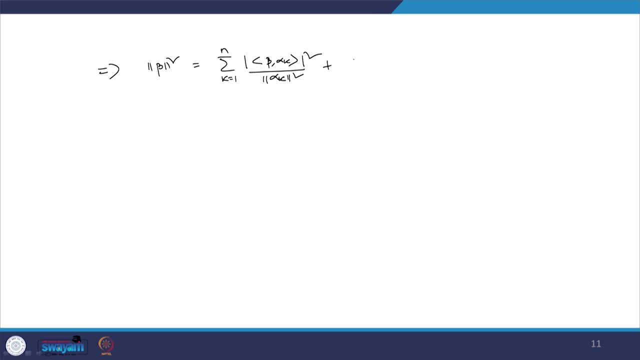 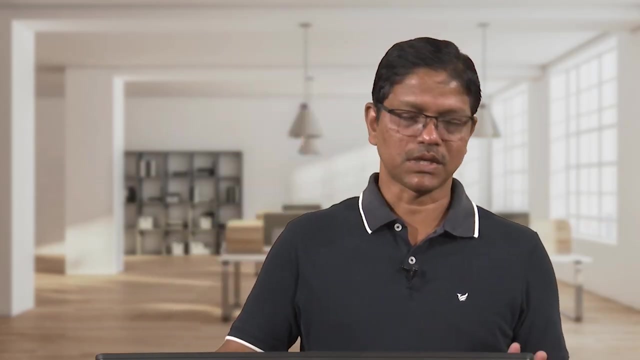 k equal to 1 to n, plus your norm of beta 2 square. ok, So this quantity is also positive quantity. So the concept of orthogonal projections gives so nice results on the inner product space. It split the space into direct sum of two subspaces and it also talk about the